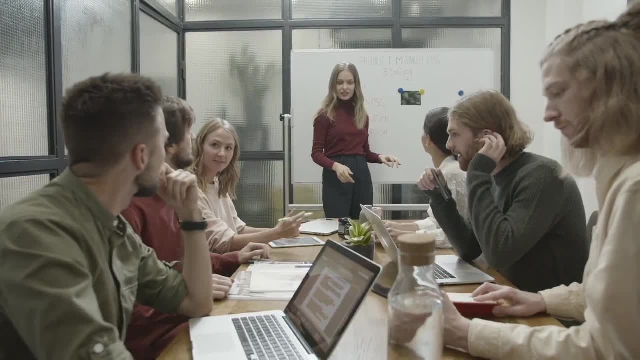 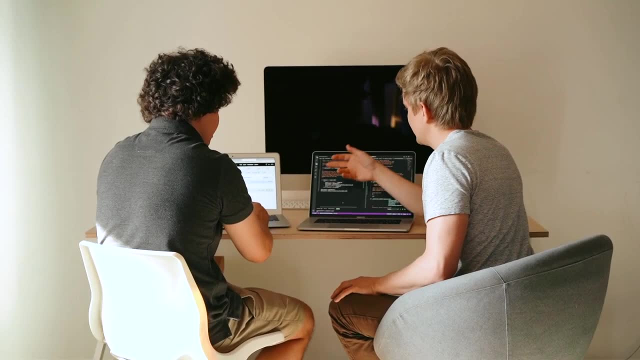 them to communicate with various engineering leads and customers, or even the sales teams. whereas the embedded software engineer focuses on the software product and usually is focused internally on that specific team, Embedded system engineers are concerned with the overall system during their entire life cycle. Embedded system engineers are concerned 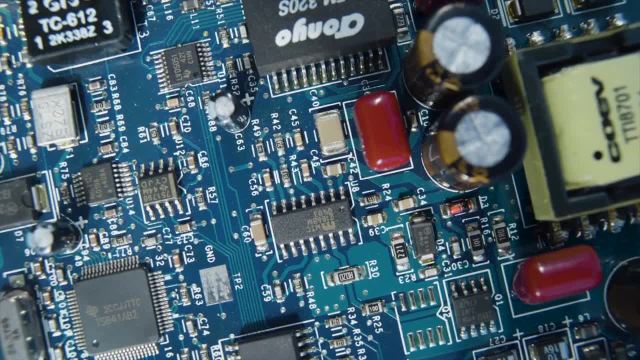 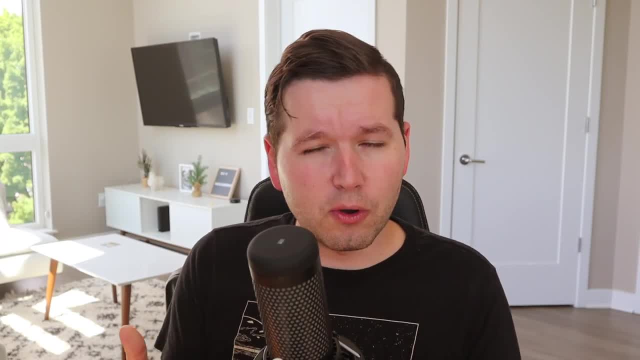 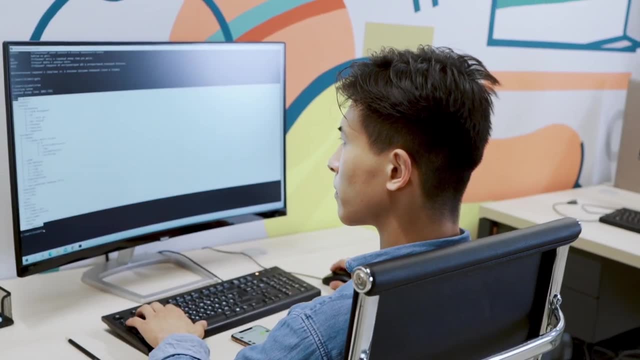 with all aspects of the system development, including hardware, software manufacturing and process engineering. Even though the system engineer focuses on the overall system, it is also pretty common for them to be involved directly with the hardware or software designs, especially in smaller companies where there is no dedicated person for each of these positions. Embedded software. 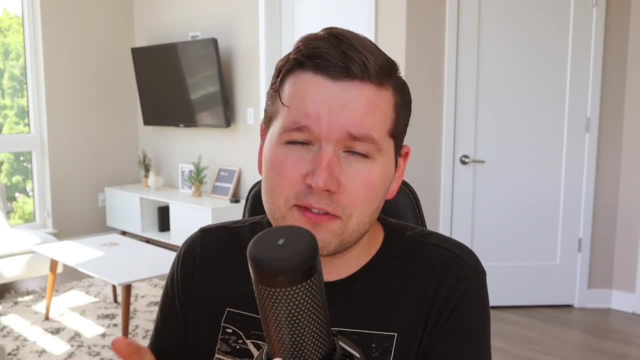 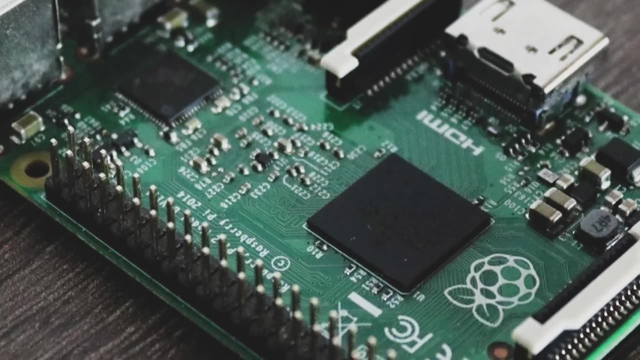 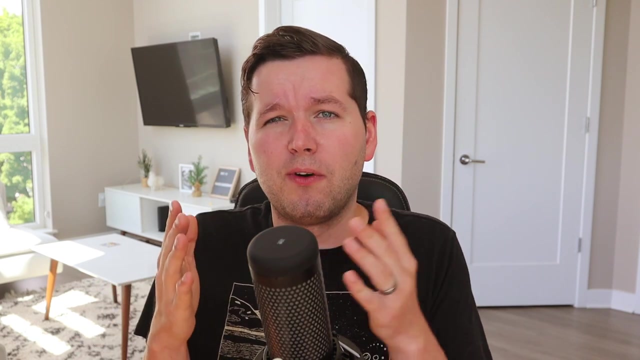 engineer typically focuses merely on this embedded software development infrastructure or anything else that they need to do to accomplish their tasks within firmware or software development. As I've mentioned in my previous videos, depending on the person and the company, embedded software engineers can be involved directly with some hardware design to some extent. 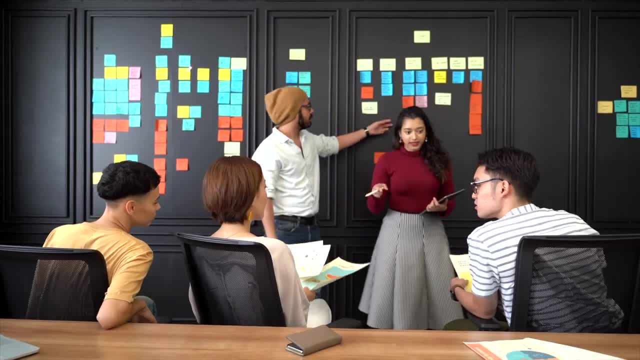 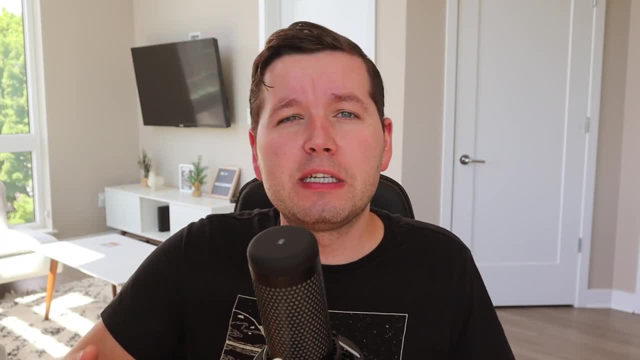 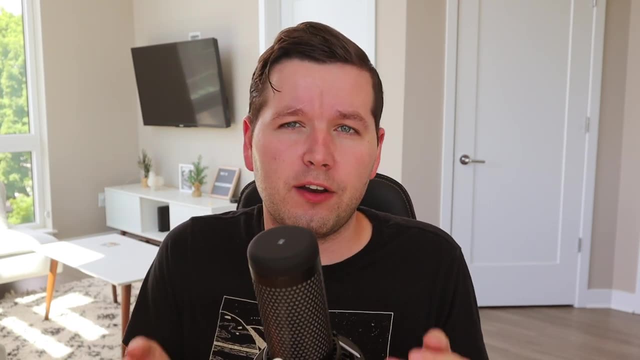 Embedded system engineers typically take marketing and customer requirements and make them into system-level discipline requirements. In this case, the embedded software engineer would be taking those requirements and looking at how it impacts the embedded software and what requirements need to be modified or created for the software itself, For example. 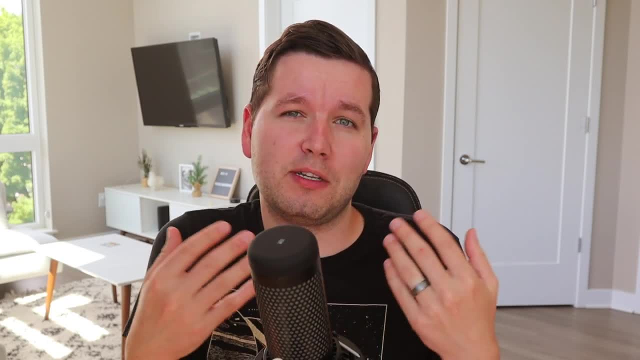 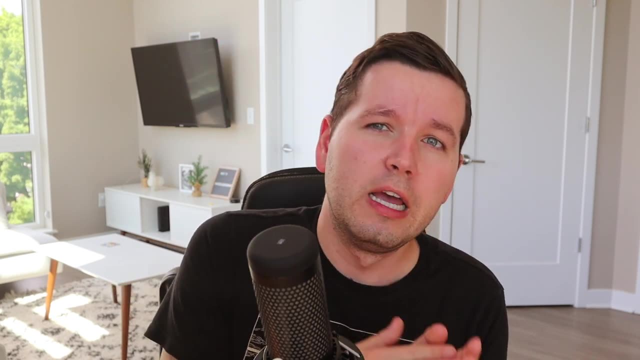 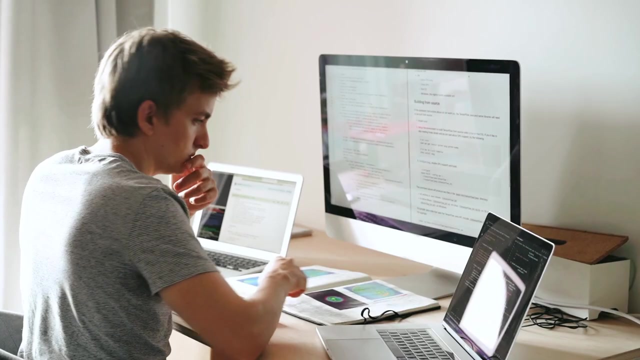 the customer wants to transfer data to their phone app, so the system engineer creates requirements around it to add the Bluetooth interface onto the product. This would translate over to the electrical engineer needing to add a Bluetooth chip on the board. Embedded software engineer would write the software to communicate with the phone itself and the software engineer. 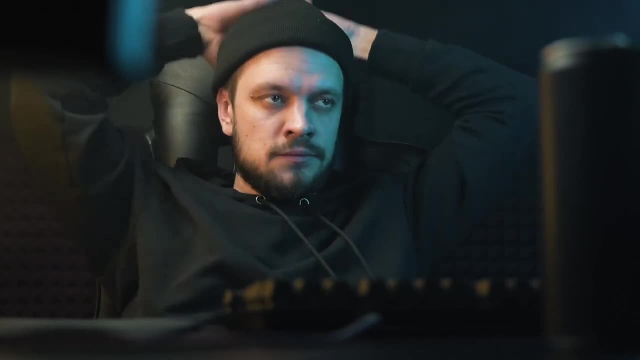 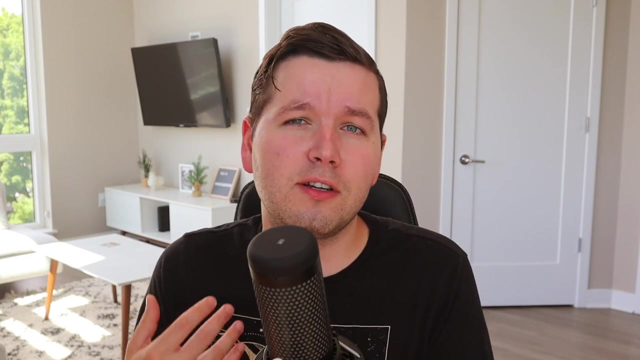 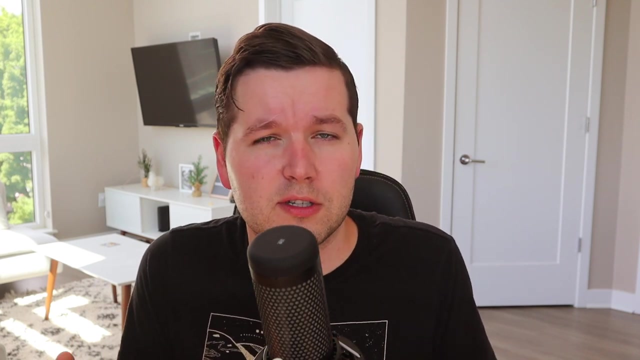 would create a phone app to essentially communicate with that product. Obviously, this is very simplified, but each of these subsections of mechanical engineering, electrical software and so on will have their own requirements of how things need to work and how they need to interact with the whole system. Honestly, I can give you all these comparisons. 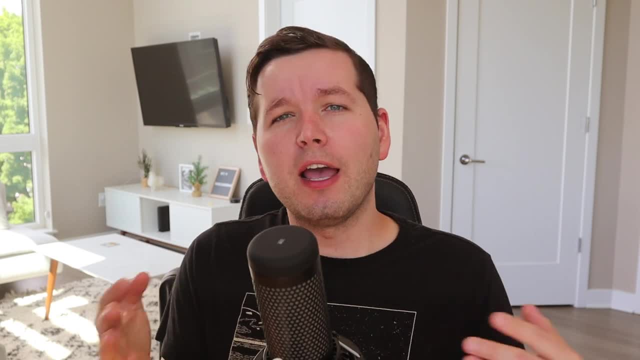 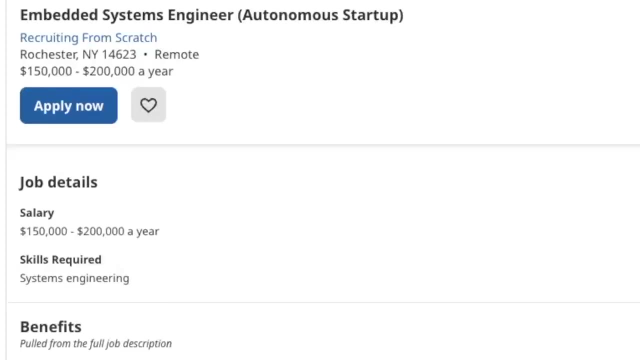 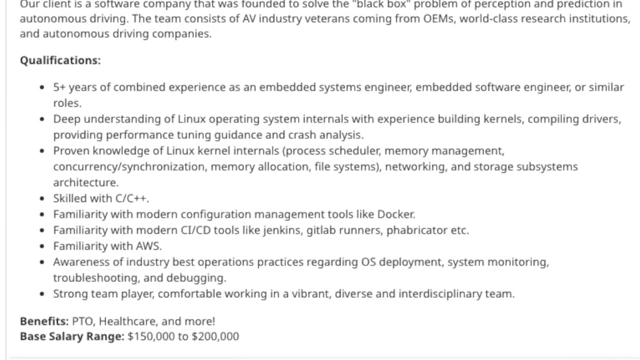 about these positions but, as I mentioned earlier, every company does things a bit different. If you are looking for a job, I highly recommend you read through the descriptions of those positions to actually understand what your responsive capabilities will be. This way, you don't have to assume what that position is about.